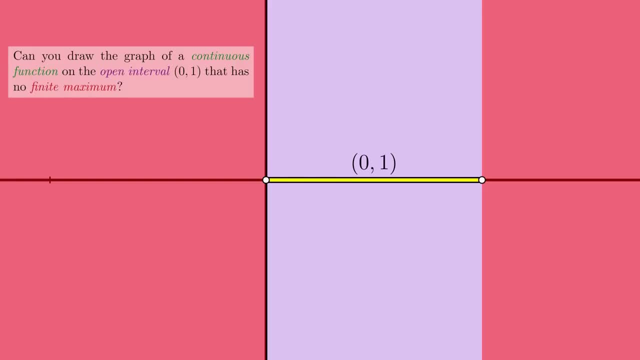 that has no finite maximum on that interval. That is, can you draw a single continuous curve moving from left to right that has no highest y-coordinate? Many of the regular kinds of curves you could draw wouldn't be able to do this. But if 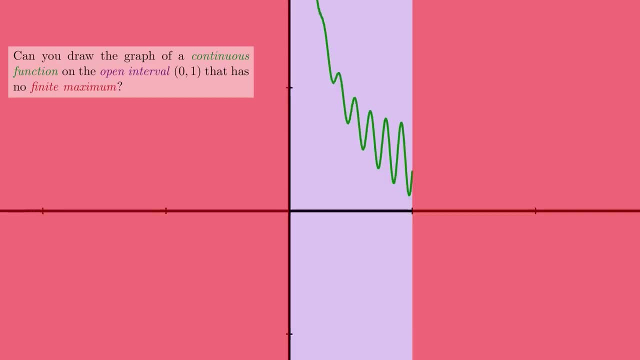 you've seen enough graphs in your life. you might have an idea. Try the function 1 over x. Its graph forms a vertical asymptote at x equals 0, meaning the height of the graph grows without bound as x approaches 0, though the graph never actually reaches x equals. 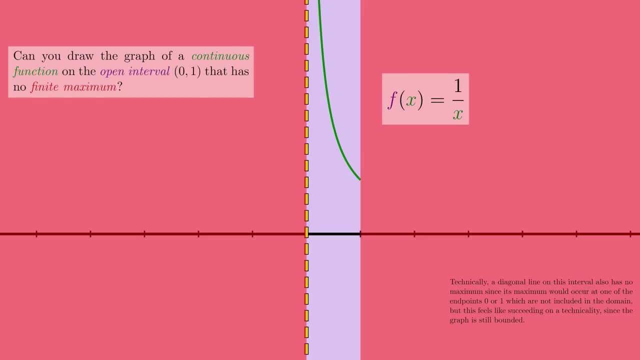 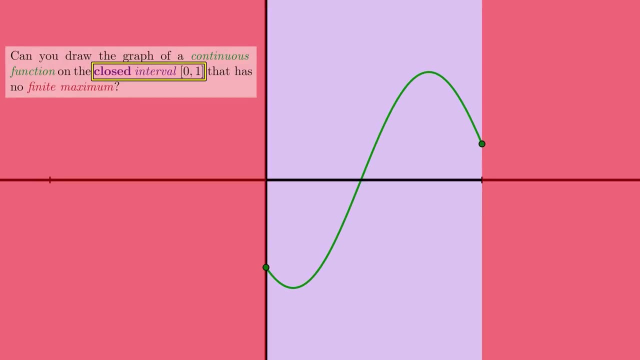 0.. Thus it has no finite maximum. Alright, but what if I require the graph to actually touch both? x equals 0 and 1? That is, the graph must actually contain a point with x-coordinate 0 and another point with x-coordinate 1, in addition to all the values in between. So no funny business with. 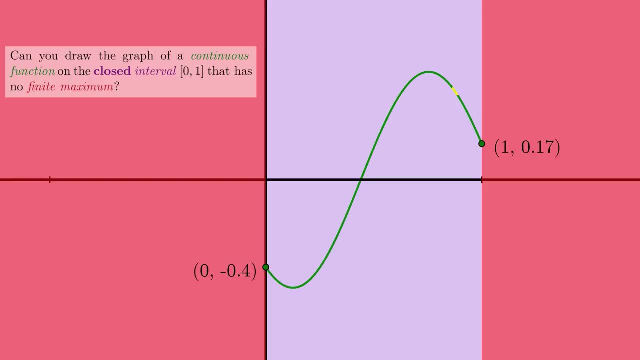 asymptotes or holes, but it still needs to be a single, continuous curve. Can you draw a curve that has no highest point? now, Not so easy, is it? It's tempting to try and fit an asymptote somewhere, but anywhere you put one will result in a discontinuity. 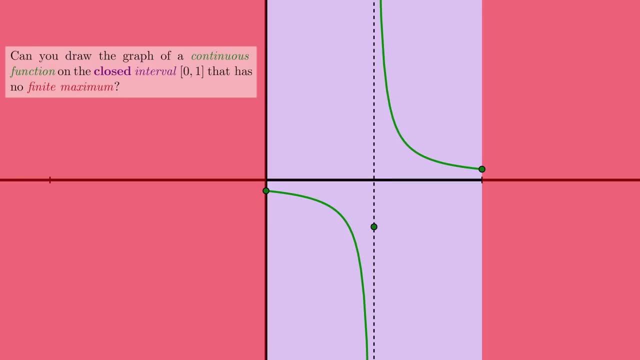 Since the function now has to be defined at the actual asymptote point itself, and we're not counting infinity as a number here. So it seems like we're forced to actually have a legitimate highest and lowest point on the graph. We can't avoid it. 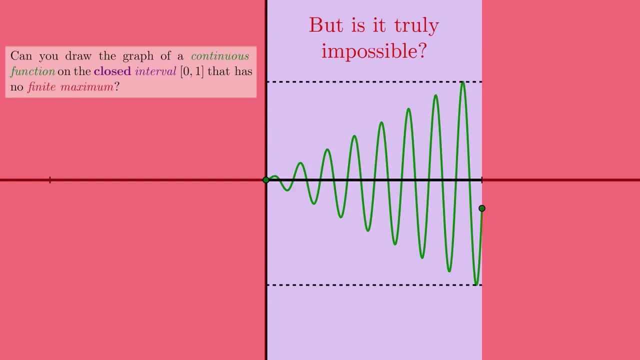 But is it actually impossible, though? How do you know? If you'd never seen an asymptote before, you might not have thought of that solution in the previous case. So how do you know? there's not some similarly clever trick that will allow the function to avoid having 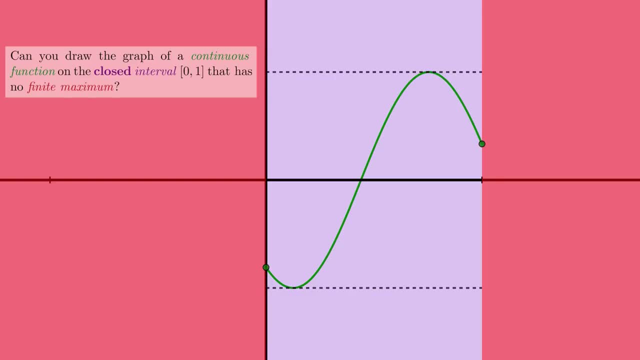 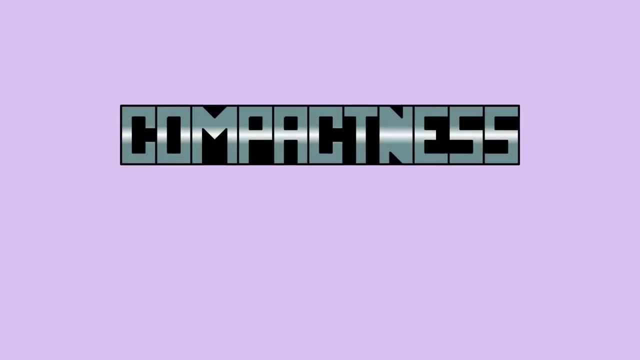 a max or a min in this case. Well, it's questions like these that the concept of compactness helps solve. It's one of the most important concepts in topology and analysis, but it can feel a little mysterious and also contrived when you first learn about it. So what is compactness intuitively, And why? 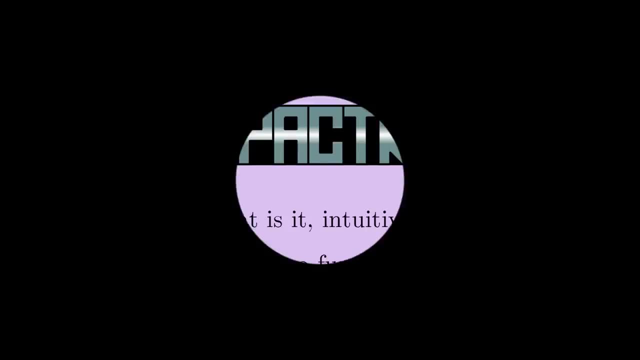 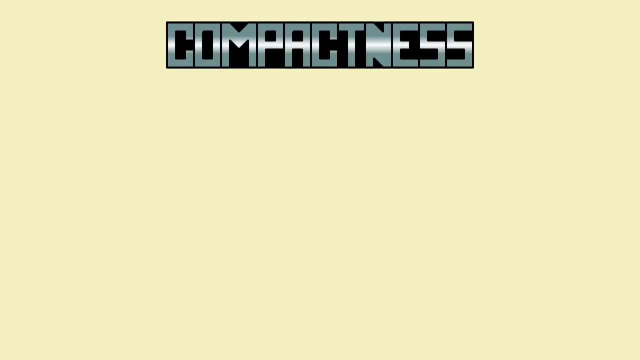 is it so fundamental to so much of modern math? Compactness is a property of shapes. Compactness, K, stands for a type of variable. it'll mean that k's and c's take total parts of k, which gives a set of points. but 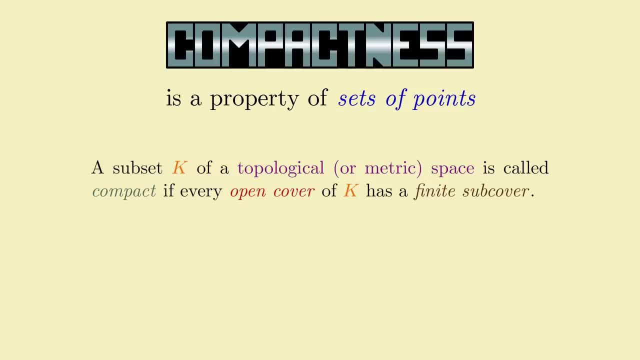 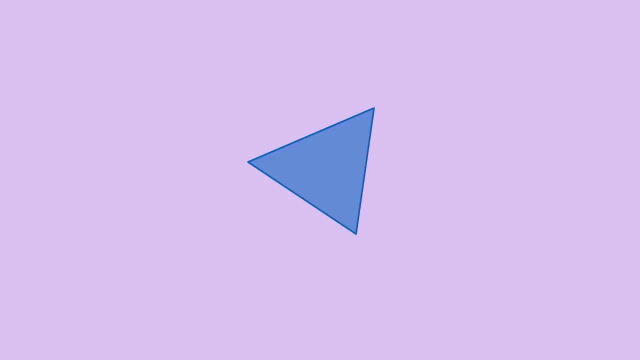 does not deny how selectively they lie. Compactness gives depth in cases, So this is a Morgan rule. Very simple topological or metric space. What is that? I went over this briefly in my video about connectedness. but just to recap, remember, in topology all shapes, curves etc. are thought. 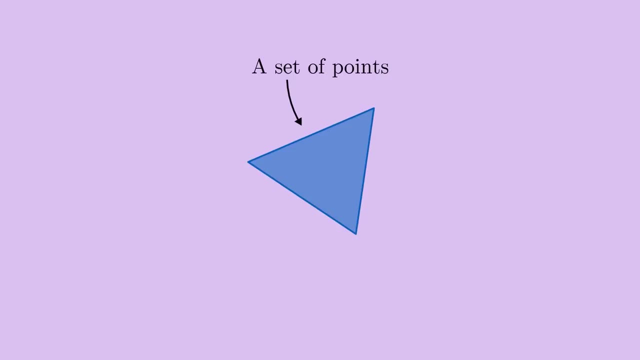 of as a collection or set of points, And any set of points S divides the space it lives in into three other sets: The interior of S, consisting of all points that can be enclosed in a ball that's also contained in S. The exterior of S, consisting of all points that 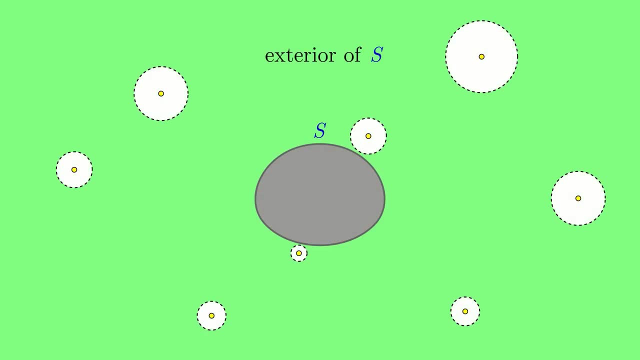 can be enclosed in balls that are completely disjoint from S. And finally, the boundary of S points where any ball containing them, no matter how small, are only ever partially inside or outside S. The critical thing to note is that a set may or may not include its boundary. 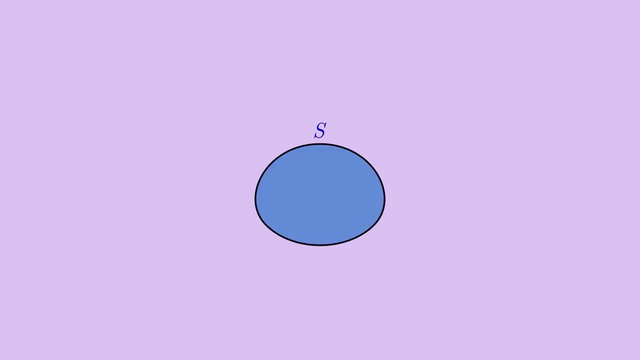 or can even include just part of it. A set that includes all of its boundary is called closed, a set that includes none of its boundary is called open, and a set that includes only part of its boundary isn't special enough to get a name. So, getting back to our definition, 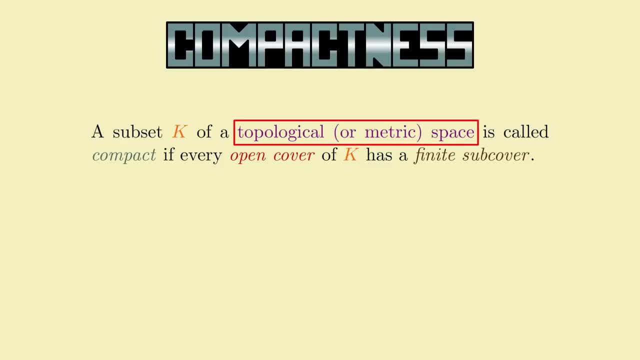 without going into too much detail, a topological or metric space is just a space where concepts like open, closed, interior, exterior boundary and so on make sense. The important sets to pay attention to regarding compactness are the open sets. Those are sets that only consist. 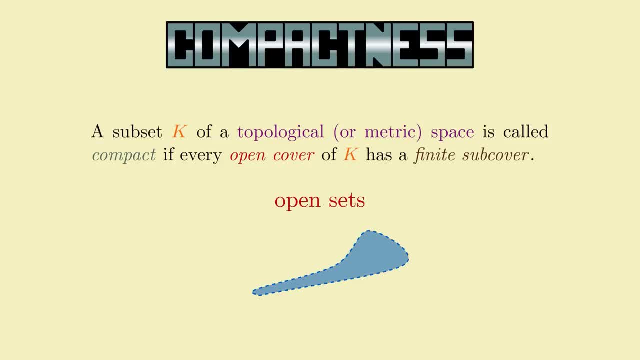 of interior points, which is important, since it means they always have to be a little bit fat, since any points inside them have to be able to be enclosed in balls that are also inside the set. This brings us to the next part of the definition: open covers. This one is pretty straightforward. 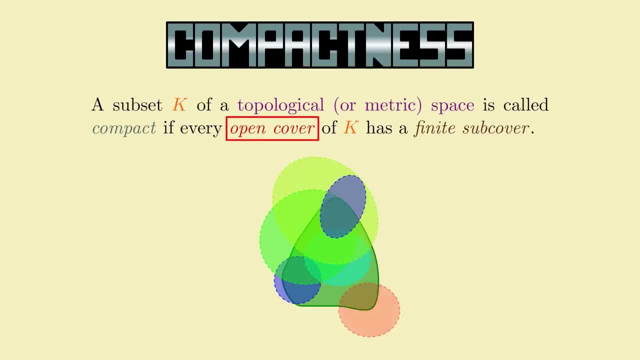 An open cover for a set is a collection of open sets that collectively cover the target set. There could be finitely many of them, or infinitely many, and can individually have any size. A sub-cover is just a sub-collection of these open sets that still manages to cover the target. 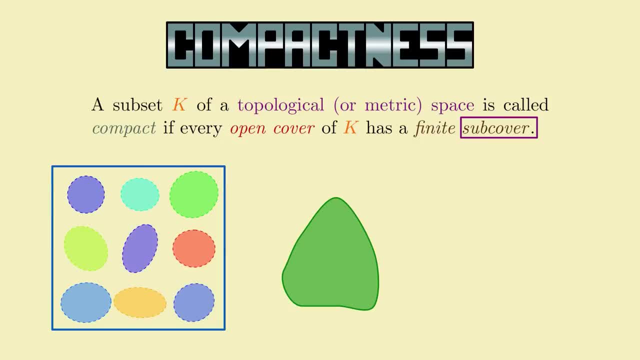 set. Note, we also include the original cover itself as one of its sub-covers. So, putting all this together, a compact set is a special set where, for any possibly infinite collection of open sets you come up with to cover the set, you can always select a finite. 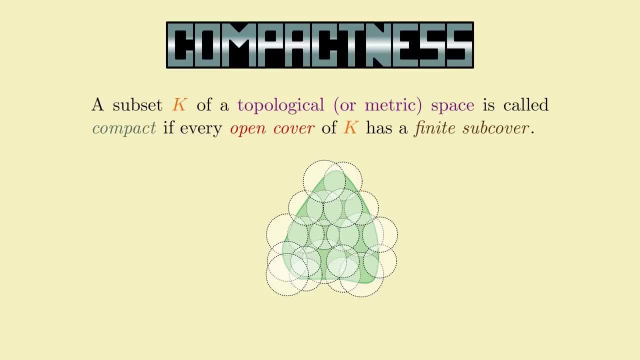 sub-collection of them that will still cover that set. Note that this isn't the same as saying the set can be a collection of open sets, but it's a collection of open sets. that can be a collection of sets that can be covered by finitely many open sets. That's actually true of all sets, Just. 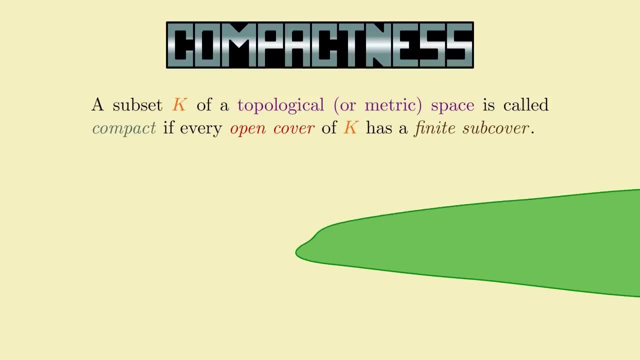 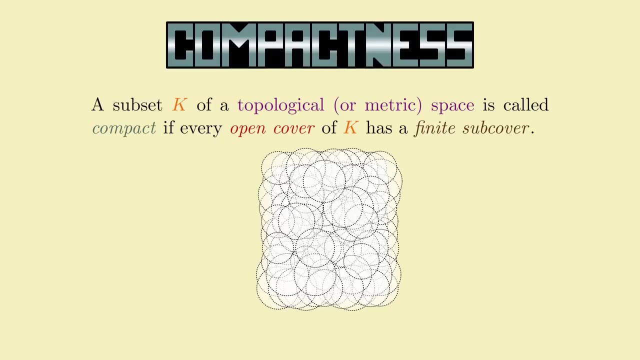 pick a big enough open ball to cover it, Or, if it's an unbounded set, just use the entire space itself, which counts as an open set. No, this is saying something more subtle. It's saying that if you give me a potentially crazy, complicated collection of open sets that covers the compact, 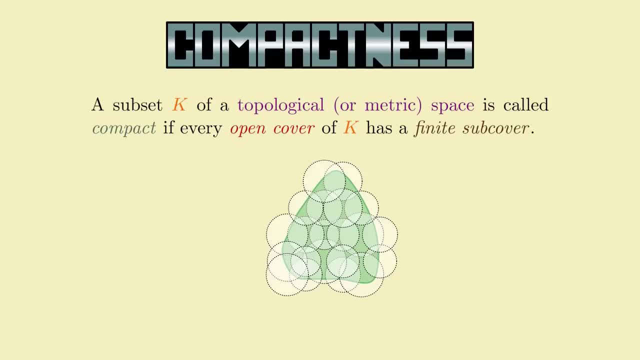 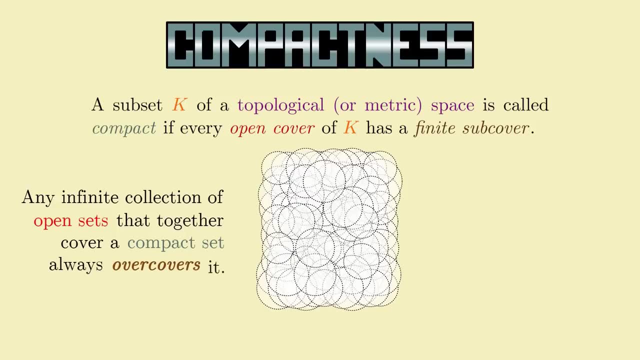 set. I can always cover the set using only finitely many of the open sets you gave me. Or to put it another way, any infinite collection of open sets that together cover a compact set always overcovers it. You can always get away with a finite sub-collection And that's it. That's all. 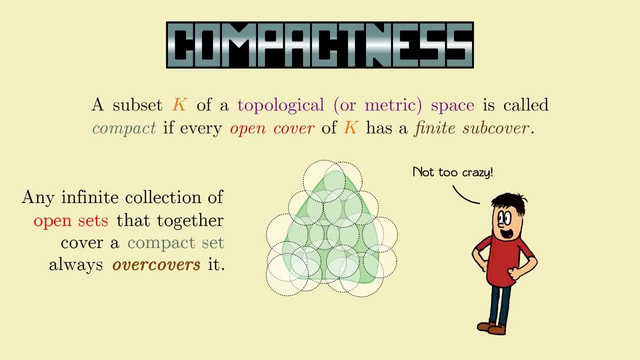 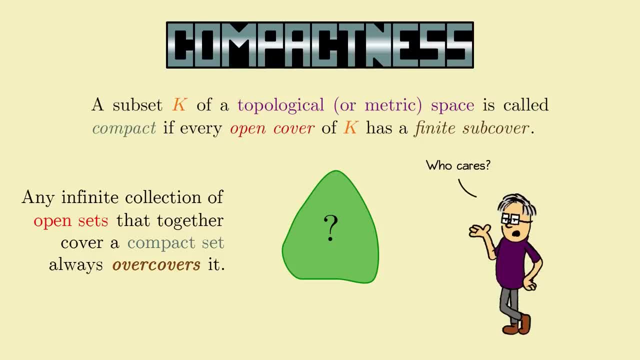 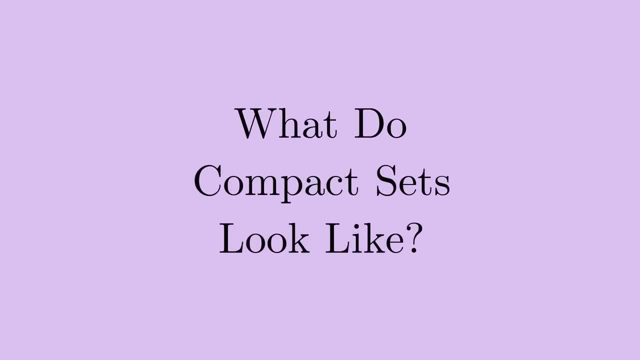 be that interesting or important anyway. So let's see if we can get a better intuitive sense of what these sets are and what they can do. The simplest kind of compact set is just a finite set, a collection of finitely many points. 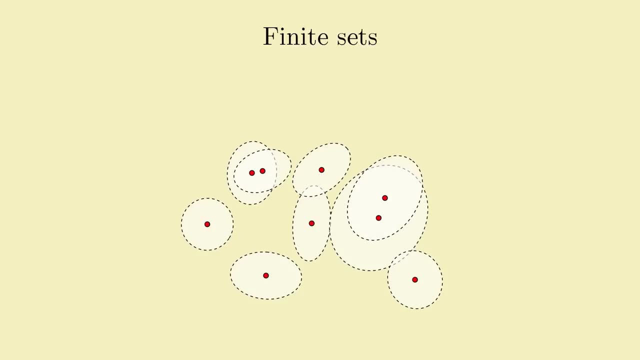 Because if I cover a finite collection of points with open set blobs, I can just go point by point and select one open set from the cover that contains it And in the end I'll have selected at most one set per point, though in practice may be fewer since some of the 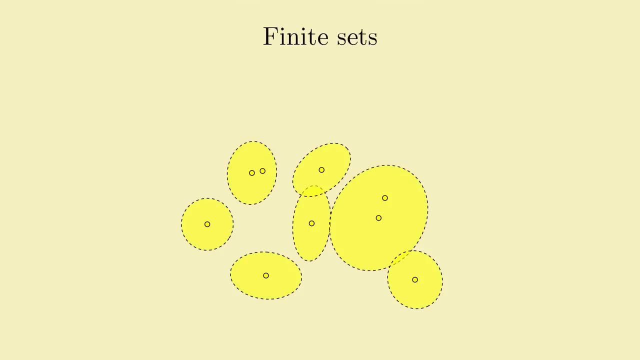 open sets I selected might cover multiple points. This actually gets pretty close to the heart of what compactness is meant to do. Compact sets sort of simulate finite sets for topological purposes, in the sense that certain tricks or techniques that work on finite sets also work on compact sets. 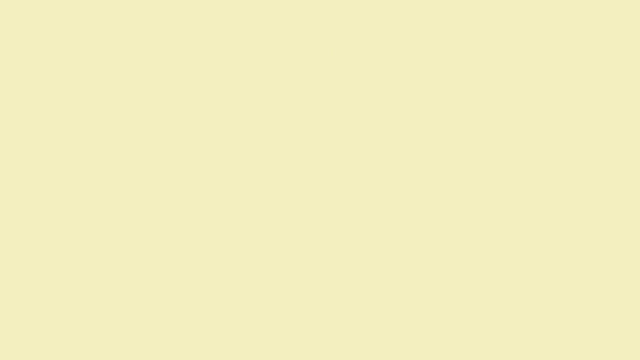 but more on that later. Beyond finite sets, the first examples of compact sets you're likely to be introduced to are closed and bounded sets of the real number line. So the closed interval 0 to 1 we saw at the beginning of the video is an example of a compact set. The fact that closed and 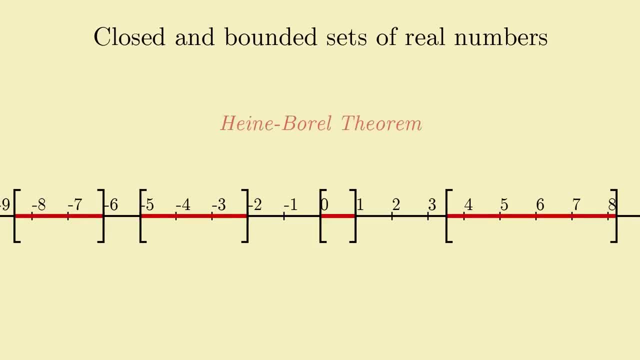 bounded sets of real numbers are compact is known as the Heine-Borel theorem and is a foundational result in analysis. I won't go through the proof of it here though, since it takes a little finesse, and I also don't think it sheds that. 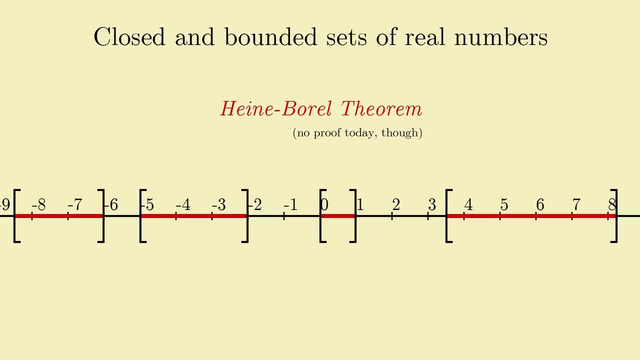 much light on the broader question of how we should interpret the real number line. If you're interested in learning more about the real number line, please subscribe to my YouTube channel and I'll see you, in the next video, interpret what compactness means. For that, I think it helps to turn to an 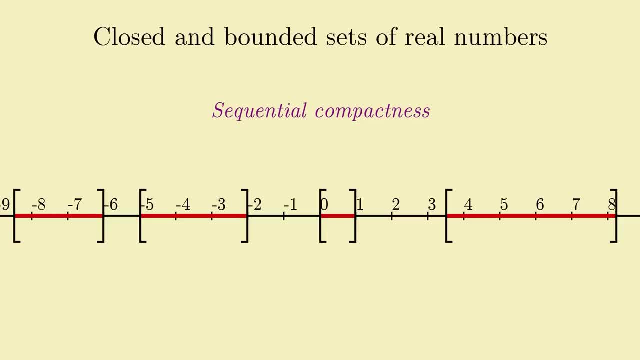 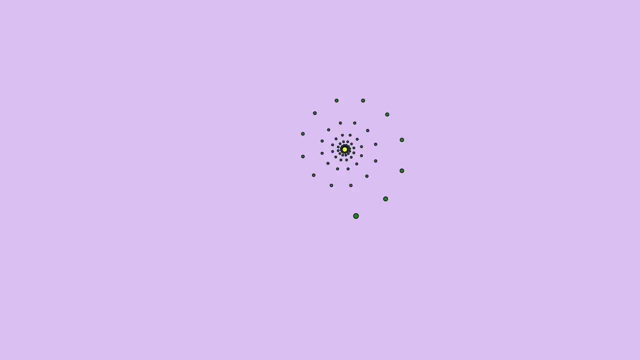 alternative description of compactness, called sequential compactness. To understand it, think about a sequence of points. Depending on the sequence, it may or may not converge toward a limiting point. If it doesn't converge, it may fail by diverging off to infinity or by wandering aimlessly around without 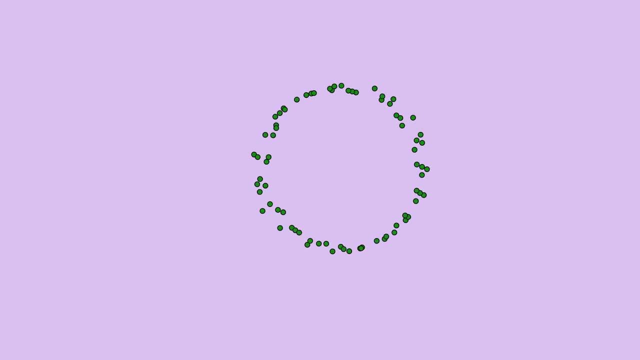 approaching anything. But in this second case, you can sometimes extract a convergent sequence out of the sequence and then convert it to the real number line. Here's an example. Consider the sequence which just alternates between zero and one. This sequence is divergent since it never makes up its mind, so to speak, about whether it's approaching zero or one. But if we selectively ignore every other term, we get a sequence that just looks like an endless string of zeros or ones, which of course converges to zero or one. 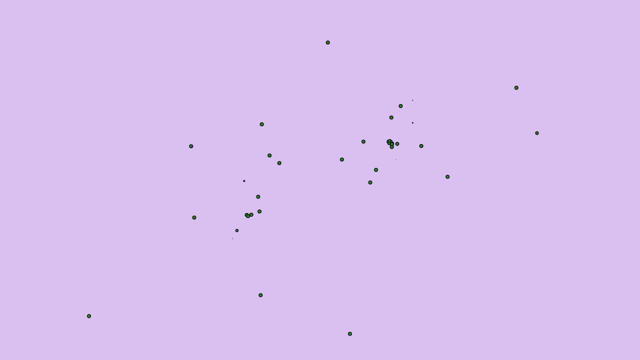 That's an extreme example, but more generally, if you have a sequence that diverges but nevertheless forms clusters in certain spots, then by carefully throwing out points not in the clusters, you can sometimes extract a convergent sequence out of it, what you might call a convergent subsequence. 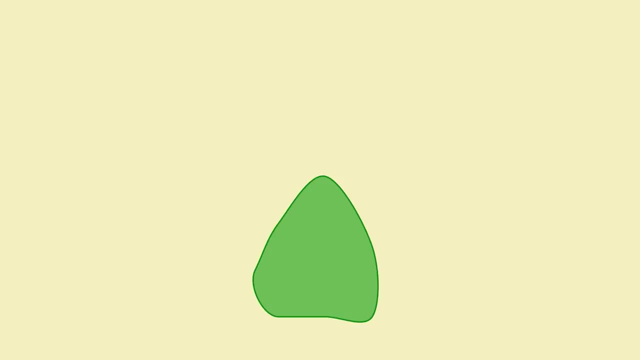 Now bringing it back to compactness. it turns out a set is compact if, and only if, every sequence of points that stays within that set, as a subsequence that converges to a point also in that set, That is a compact set is a set which forces any sequence of points within it to form clusters. 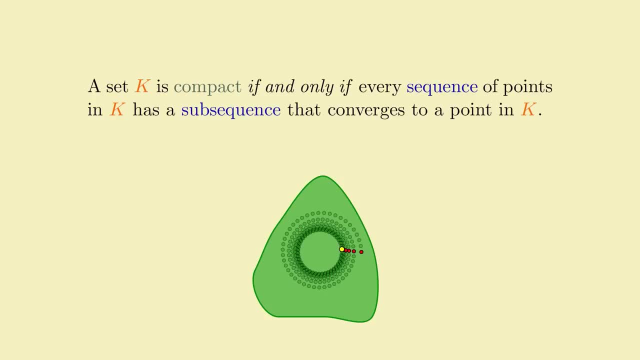 that converge toward a point, also within the compact set. This is called sequential compactness, and it's equivalent to the standard notion of compactness, except in certain more unusual topological spaces, which we won't worry about here. From this new perspective, we can perhaps get a sense for how to intuitively think about. 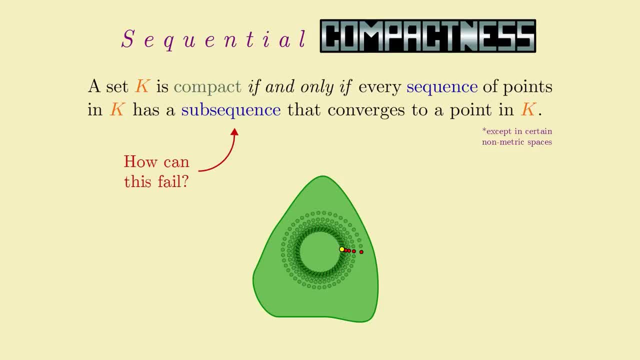 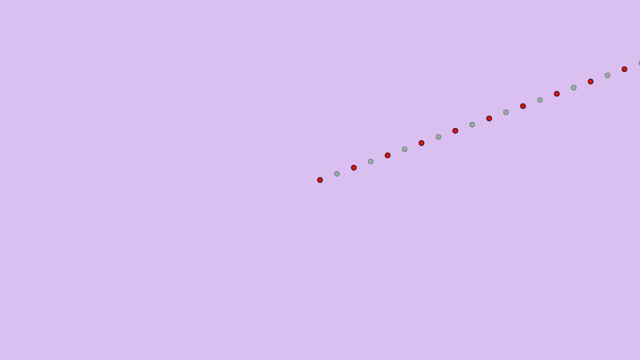 compact sets by studying the different ways a set can fail to be sequentially compact, Or in other words, the different ways to prevent a sub-sequence from converging. The simplest way is just to have the original sequence diverge off to infinity. Then any sub-sequence will also diverge to infinity, meaning any set containing such 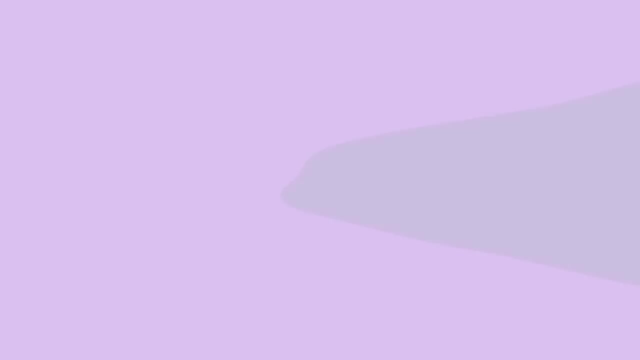 a sequence won't be compact. So the first requirement of a compact set is that it should be bounded. It can't be infinitely big or elongated. The second way to stop a sequence from having a convergent sub-sequence is to have it approach. 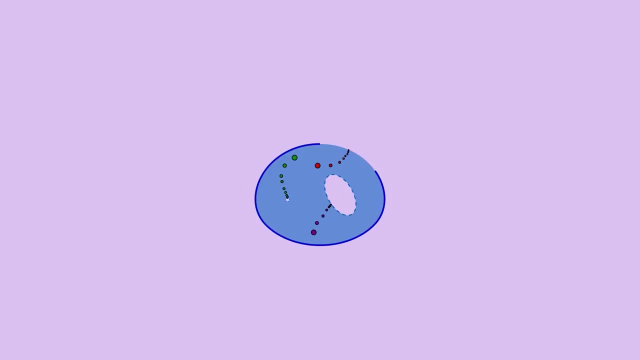 a hole or a missing point in the set, Which could either be a gap in the interior of the set or a missing boundary, Then every sub-sequence will also approach that hole and will fail to converge. So the second requirement for a set to be compact is that it should not have any such 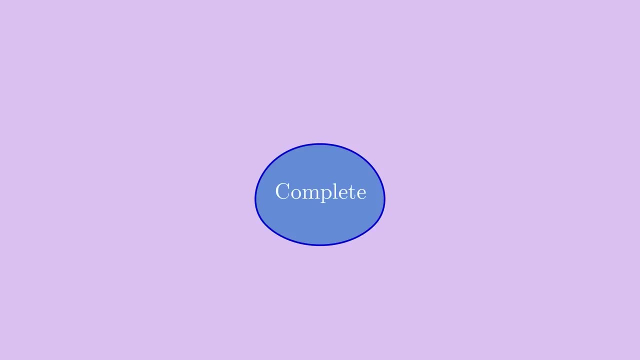 missing points. It should be complete. Now a sequence has a preponderance of boundedness and completeness. It might seem like we've covered every failure case, But there is actually a third, very subtle way a sequence can avoid having a convergent. 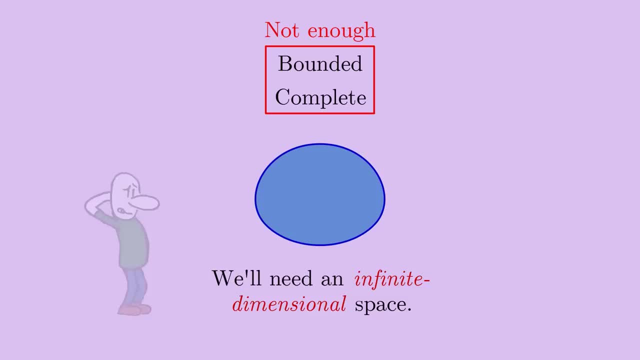 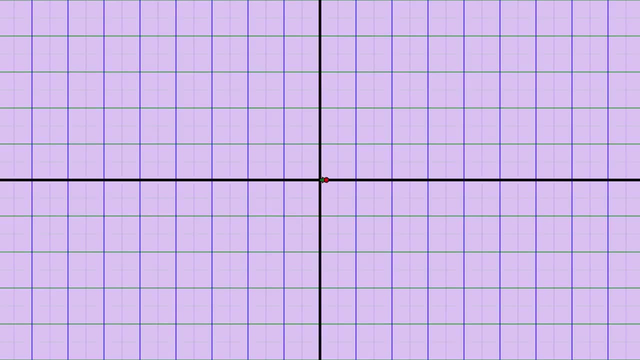 sub-sequence, But to see it we'll need an infinite dimensional space. That may sound intimidating, but there are actually some relatively simple examples. Think about it this way: Any point in a two-dimensional space can be described with two numbers: x and y. 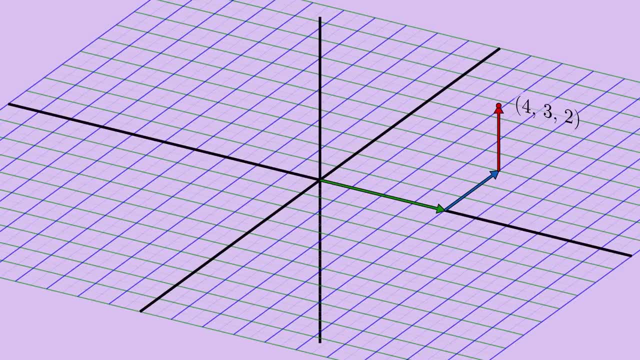 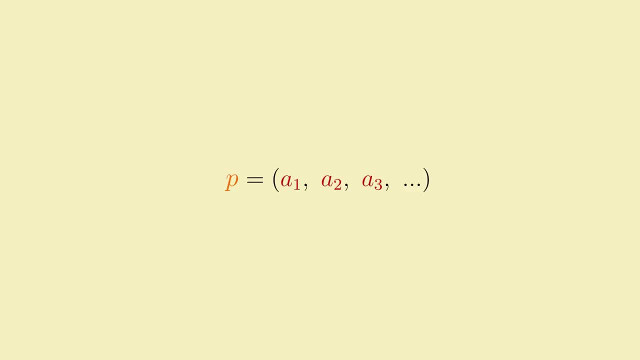 dimensional space can be described with three numbers: x, y and z. So a point in an infinite dimensional space can be described with an infinite list of numbers: a1,, a2,, a3, and so on. To keep things a little simpler for this example, I'll restrict the space to only include lists. 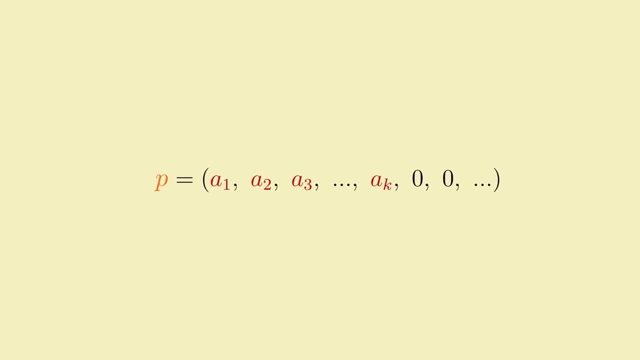 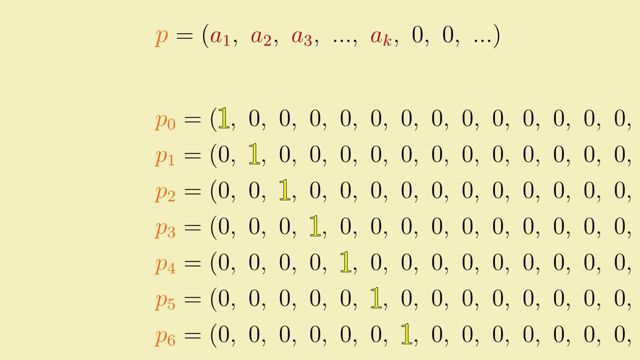 that eventually end in an endless string of zeros. With this in place, consider this sequence of points, which are actually lists. Each list contains only a single one, surrounded by nothing but zeros, where the nth list in the sequence has a one in the nth place. 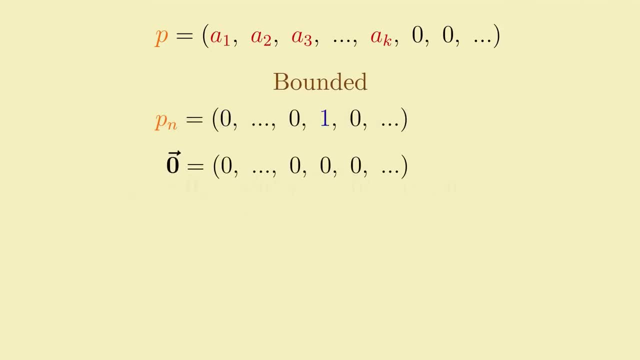 This sequence of lists is bounded. All of them are a distance of one away from the zero list, But it doesn't converge. This sequence of lists doesn't approach any list. You might think it converges to the zero list since any particular slot in the lists. eventually, 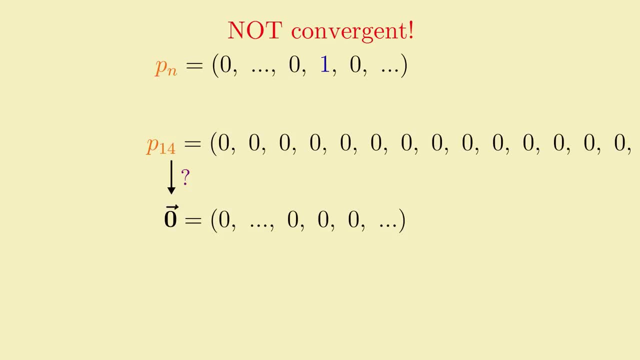 becomes a zero, But from a strict topological point of view it doesn't approach the zero list, since any list in our sequence stays a distance of one away from the zero list And naturally any sub-sequence will suffer the same fate. 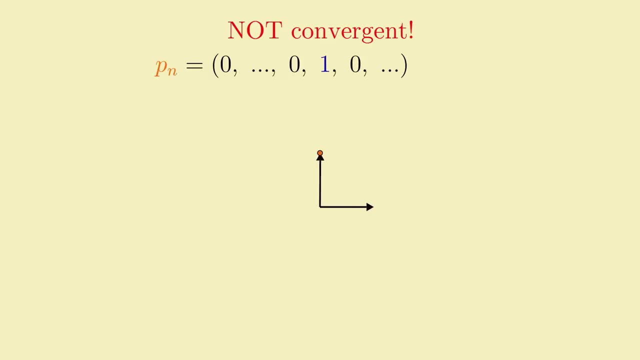 In effect, we have a sequence of points that endlessly explores all the infinitely many coordinate axes of the infinite dimensional space, while always staying a fixed distance away from the origin. So it avoids approaching anything by kind of traveling through infinite, infinitely many dimensions. Sounds like bad science fiction, but it's true mathematics. 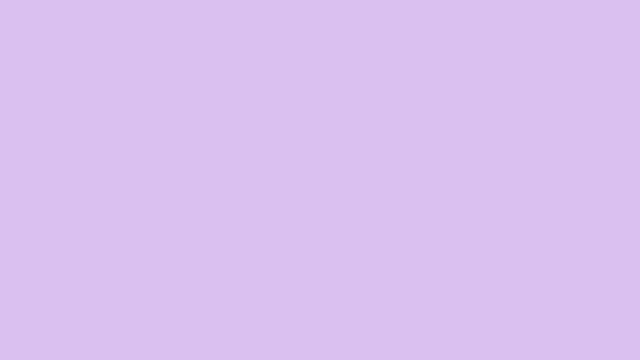 The requirement we'd need to impose on a set to prevent this is called total boundedness, and it basically says that your set can be covered by a finite number of balls of any given fixed size. In our familiar finite-dimensional Euclidean space, this is the same as just ordinary boundedness. 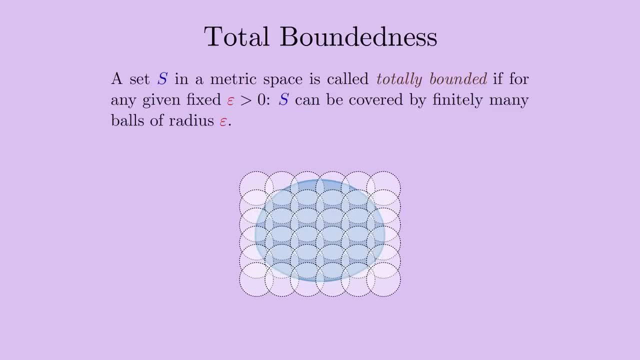 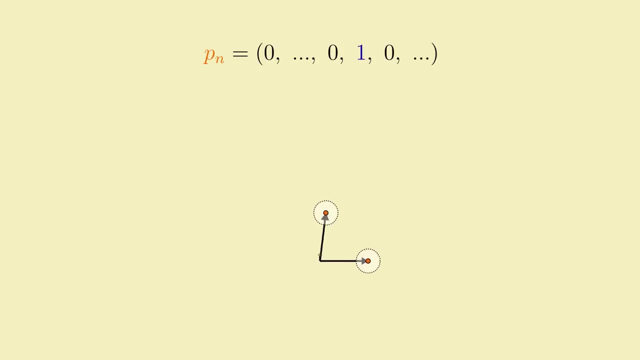 since any bounded blob can always be covered by finitely many balls of any fixed size. It may take a lot of them if they're really small, but it's always a finite number. Not so for our infinite-dimensional set, though, since if I surround each point in our sequence, 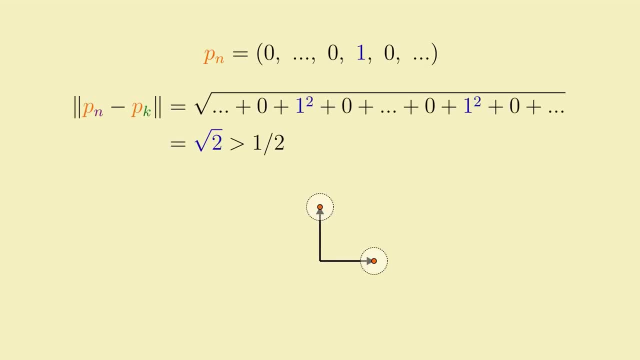 with a ball of radius one-fourth. all the balls will be disjoint from each other, since every list in the sequence is a distance of more than one-half away from every other list. So the set this sequence of lists lives in would not be totally bounded. 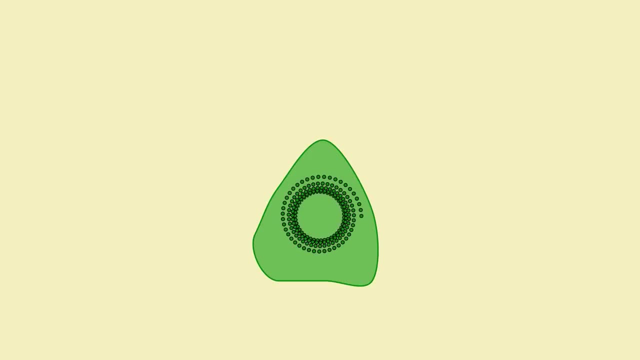 With total boundedness in place, we've finally actually got enough to force every sequence in a set to have a convergent sub-sequence. That is to be compact, Because there's a theorem that says a set is compact if, and only if, it is complete and 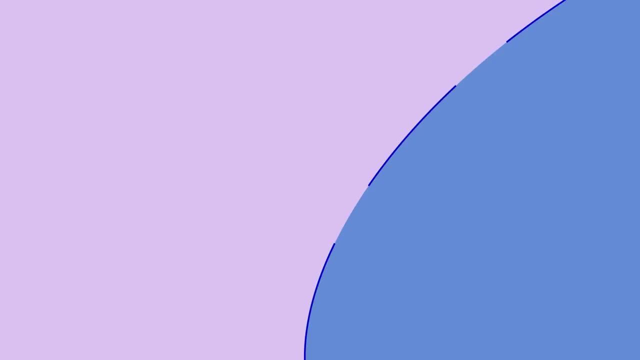 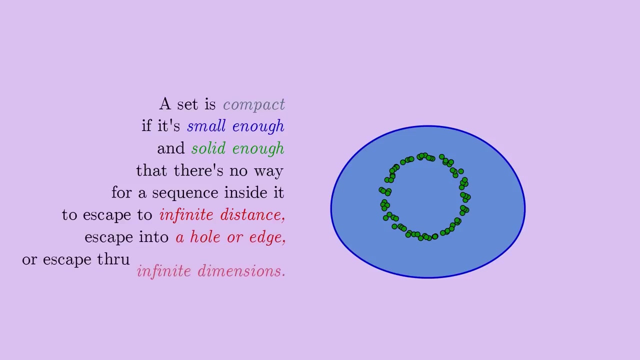 totally bounded. So this is how I like to think about compactness. intuitively, A set is compact if it's small enough and solid enough that there's no way for a sequence inside it to escape to infinite distance, escape into a hole or edge, or escape through infinite dimensions. 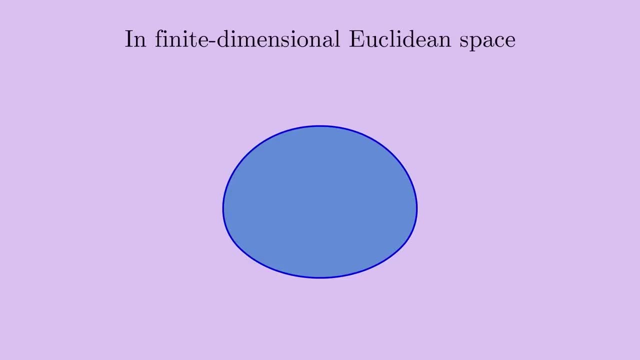 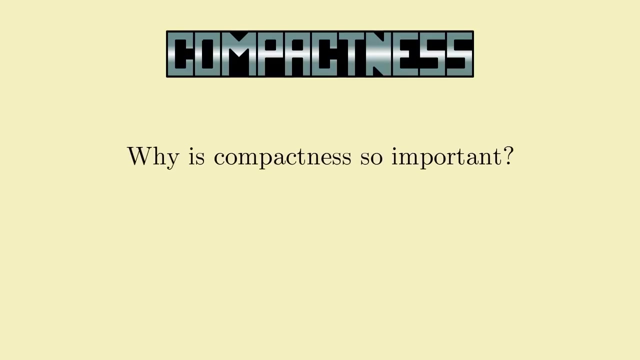 In ordinary finite-dimensional Euclidean space this corresponds precisely to the sets that are closed and bounded. But as we saw, that's not always enough for more exotic spaces. So that's how I view compact sets intuitively. But even so, why are such sets so important to analysis and topology? 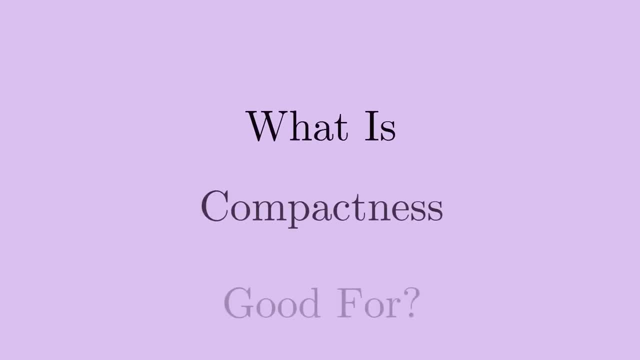 What do they let us do? Let's look into that now. One of the main reasons compact sets are so nice is they often provide a way to take properties that hold locally on the set and extend them to apply globally on the entire set. 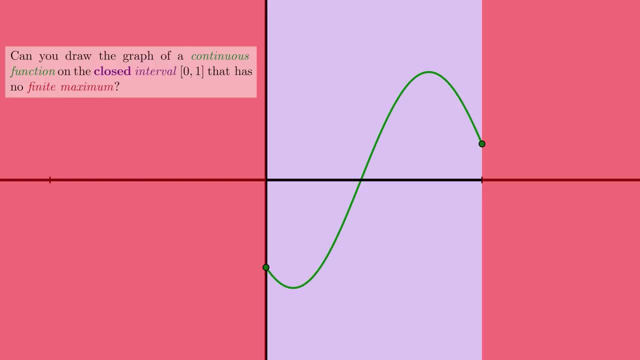 That may sound a little vague, so let's do an example. Remember the puzzle at the beginning of the video where I challenged you to find a continuous function on the closed interval 0 to 1? that didn't have a maximum. Well, it turns out it is indeed impossible, and it comes down to the fact that the closed 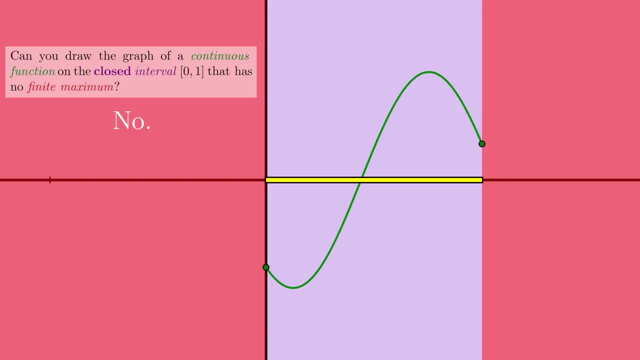 interval 0 to 1 is compact. Every continuous function defined on a compact set attains both a maximum and a minimum. This fact is known as the Extreme Value Theorem, And to show how compactness plays a key role, we'll prove a slightly weaker version of it. 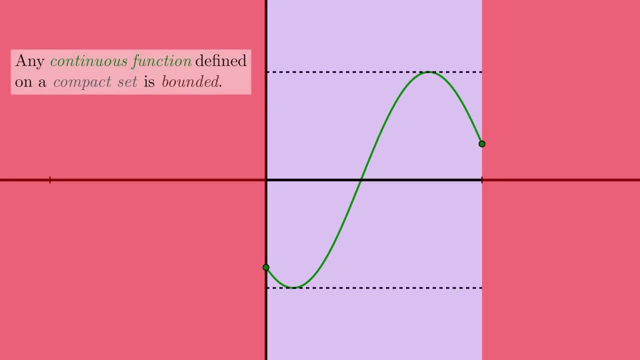 that any continuous function defined on a compact set is bounded, meaning the function's limits have both a finite upper bound and lower bound, but we won't require the function to actually reach those bounds. Just so we have something concrete to look at. let's take that compact set to be the 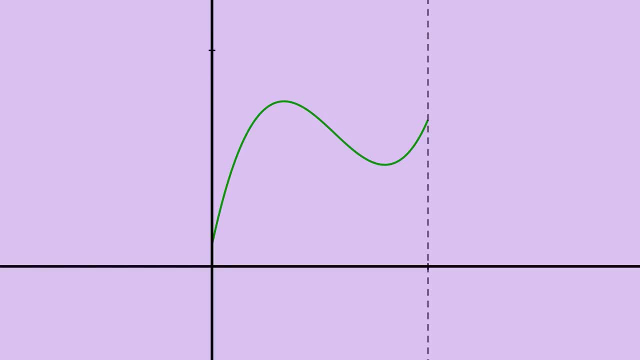 closed interval 0 to 1.. To begin, consider an arbitrary real number, x, in the interval 0 to 1.. Since our function, f, is continuous, it loosely means small changes in x result in relatively small changes in f. In fact, if I restrict the variability of f to x, the function will not be able to reach. 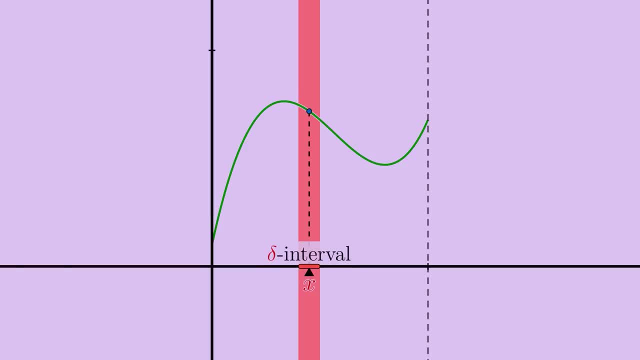 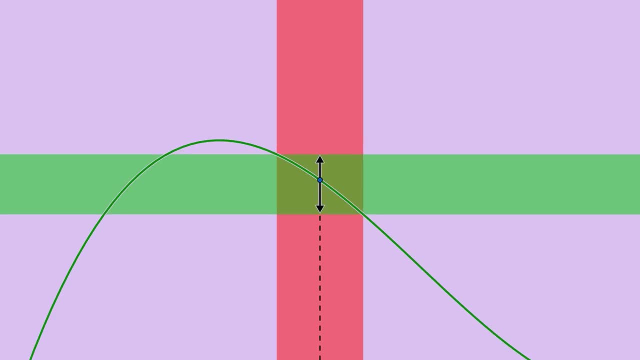 it. If I restrict the variability of x to a small enough interval- call it a delta interval- I can force the function's outputs f, to stay within certain bounds, like I dunno: a distance of 0.1 from where it started. 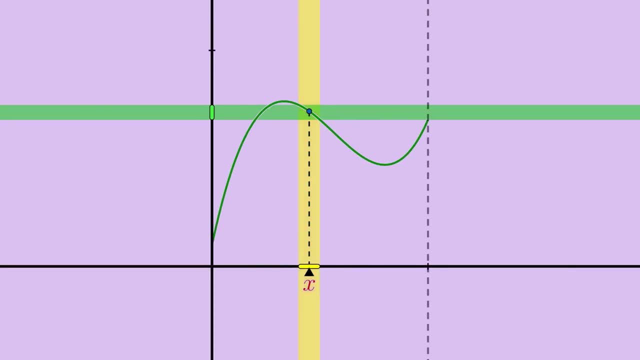 So in essence, I've defined a certain open interval around x, where the image of that interval after applying f to it, results in a bounded interval in the output space. In other words, f is bounded locally around x. Can you see where this is going? 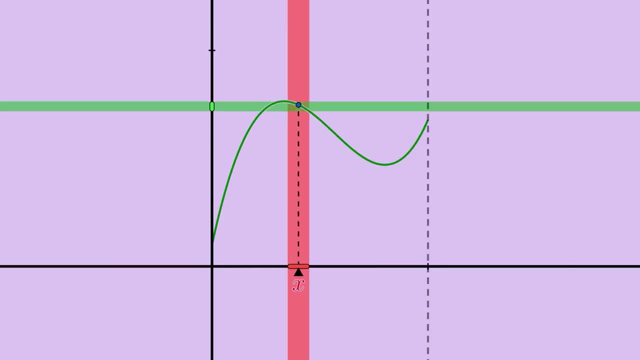 We can construct one of these little delta intervals around every single point x in the domain, creating potentially an uncountably infinite collection of delta intervals that together cover the domain 0 to 1.. But since the domain 0 to 1 is compact, it means we've over-covered it, and so we can. 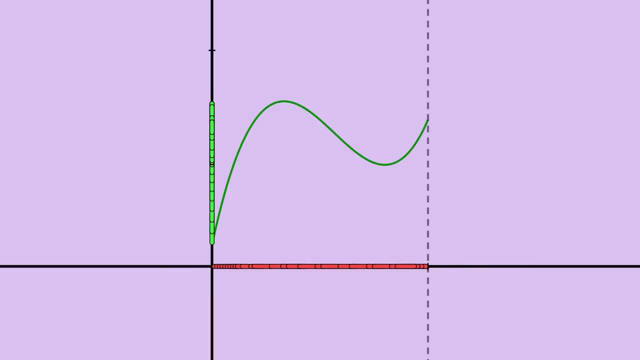 reduce down to a finite subcollection of these delta intervals that still cover all of 0 to 1.. By construction, the function f is bounded on each of these remaining delta intervals And since there are only finitely many such delta intervals, there must be a finite overall. 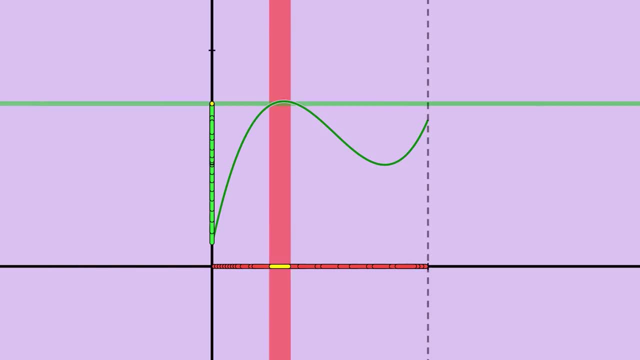 upper bound for f. Just take the highest upper bound for f among all the remaining delta intervals and likewise we can find a finite overall lower bound. Thus f is bounded on the entire interval 0 to 1.. We've taken local boundedness and turned it into global boundedness. 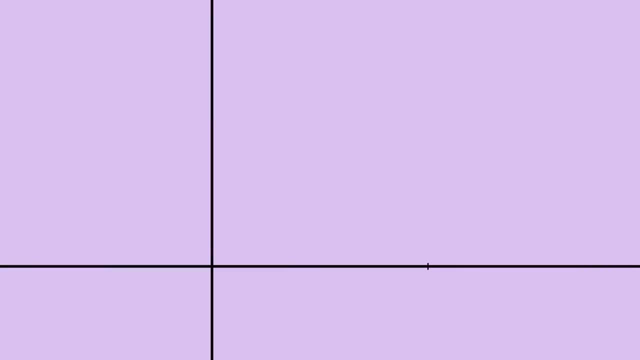 But notice how this proof falls apart if the domain isn't compact, like on the open interval 0 to 1.. If we try the same trick here for the function f equals 1 over x, we'd find the delta intervals for the x-values get thinner and thinner the closer we get to x equals 0, in. 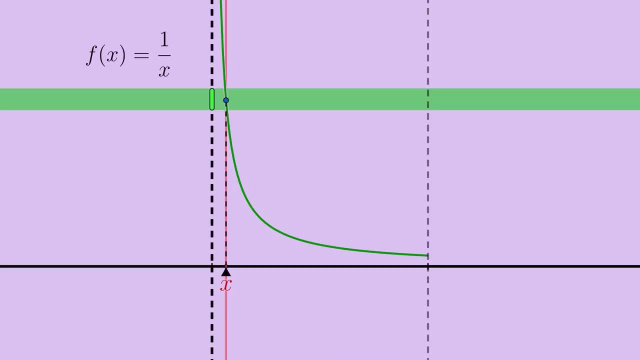 order to keep the same local bounds on y, since the function is so steep there. It doesn't take much variability of x to get y to vary 0 to 1. It's just a matter of how many delta intervals there are. It's just a matter of how many delta intervals there are. 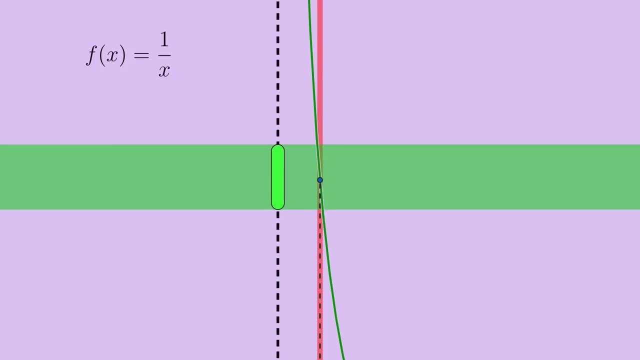 Without limiting these delta intervals to trong or beyond our maximum chosen tolerance. And here there'd be no way to reduce to a finite subcollection of these intervals, since we'd truly need an infinite number of them to cover the interval all the way down to x equals 0, since they'd be getting thinner the closer we get. 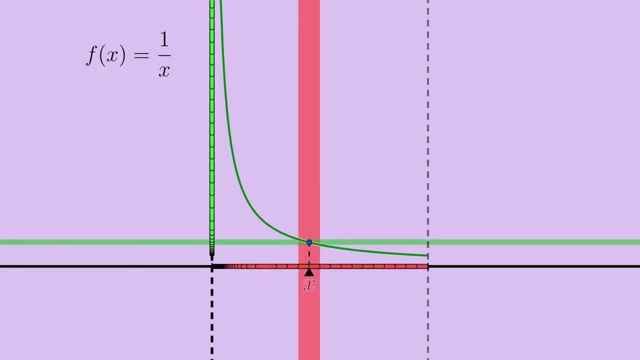 And if there are infinitely many delta intervals, we can't guarantee that there is a single delta interval that yields the highest possible upper bound for the function f and for the function one over x, Informing delta intervals that consider all delta intervals that yield the anyways of a single delta interval. we have no guarantee of how much delta intervals. 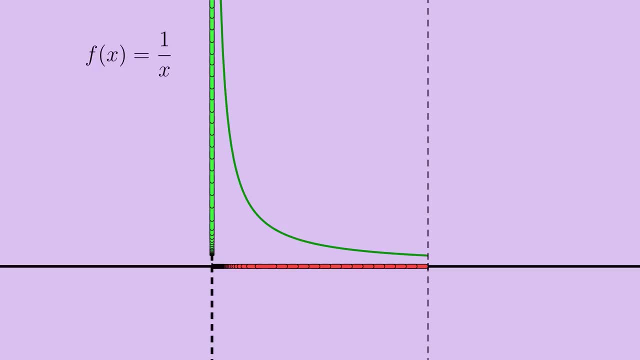 will be equal to for the function f. The point here would be to take all the willingly Wilson integrals and for the customization, for specifically there definitely isn't one. That's an overview of what compactness is and why it's so important and useful. 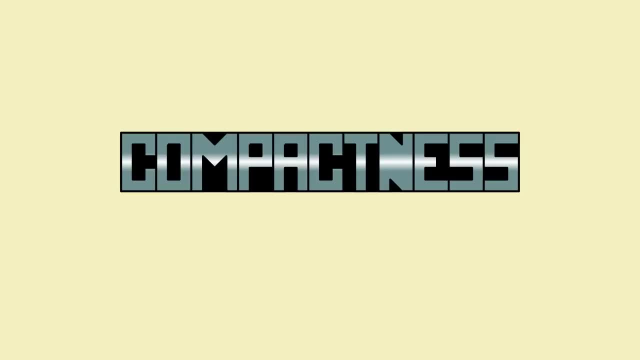 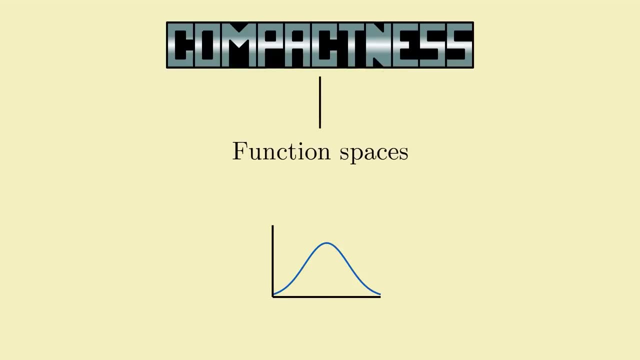 Indeed, you'll encounter the concept over and over again in higher math, where it tends to be an important ingredient in enabling many powerful constructs, such as function spaces, where functions can be treated like infinite-dimensional vectors and studied as such. According to some, being able to understand compactness might even make the difference. 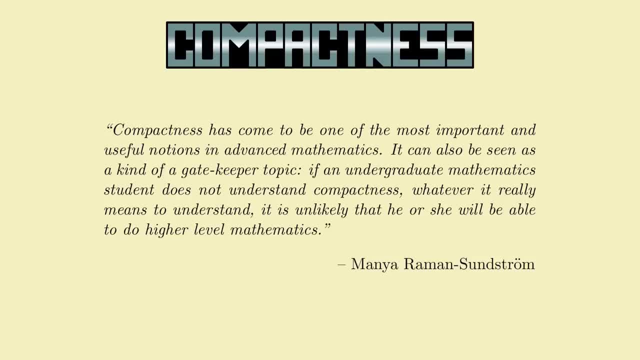 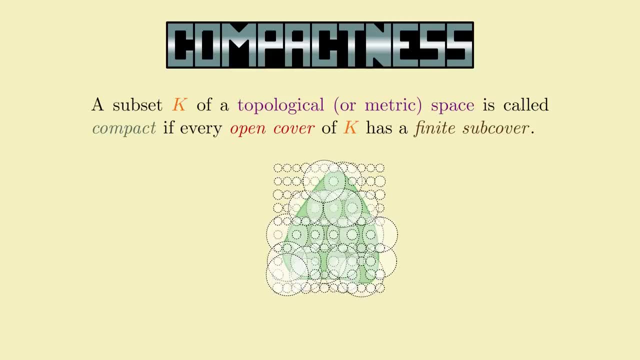 in being able to participate effectively in higher math. Much of modern math is built on compactness And if that's true, I hope this video has made it a little more accessible. But speaking of making math more accessible, one of the best resources I've encountered- 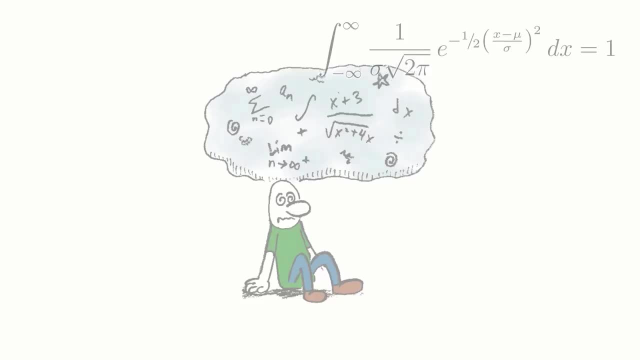 for providing a thorough and enjoyable way to learn math is this video's sponsor, Brilliantorg. One of the main applications of compactness is in the rigorous study of probability, And if you need a way to learn or brush up on compactness, you can do so by using the. 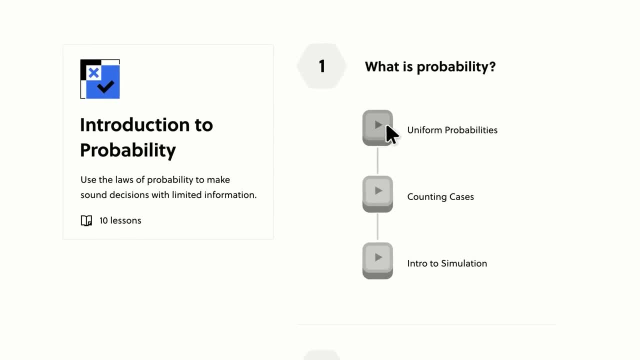 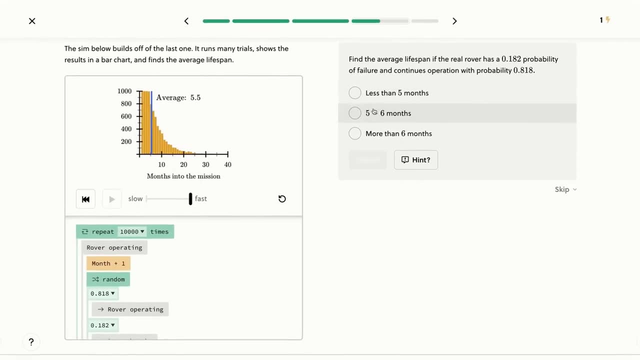 link in the description below. Brilliant offers several courses on it featuring their signature interactive lessons, Like their Intro to Probability course, which I like a lot as they have you build and run simulations right in the lesson, helping you get a real visceral feel for how it all works. 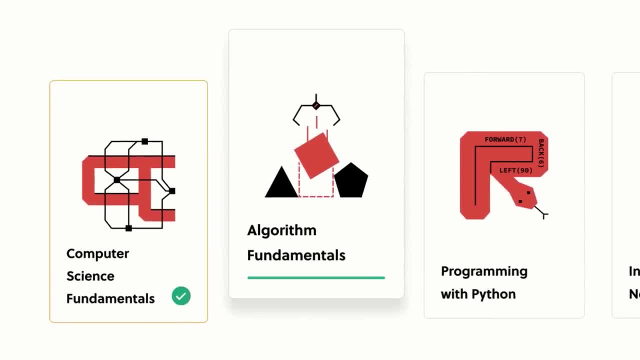 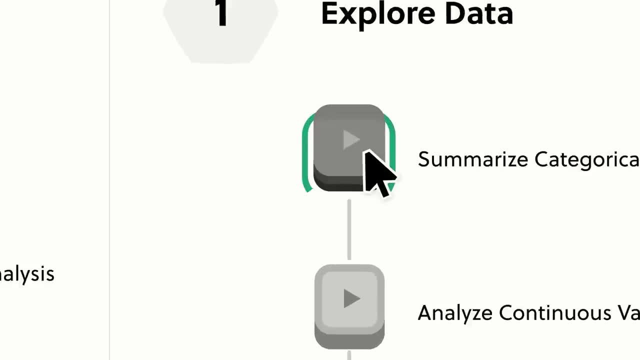 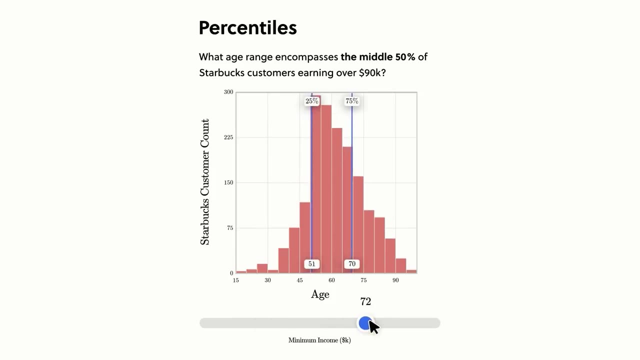 beyond just the theory, Beyond probability, Brilliant has a wide selection of thousands of other lessons in math, computer science and data science, with new lessons added every month, covering both basic and advanced topics. And Brilliant goes out of their way to make sure each lesson feels friendly, fun and